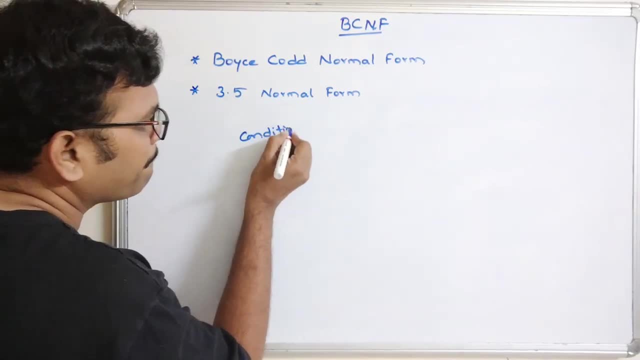 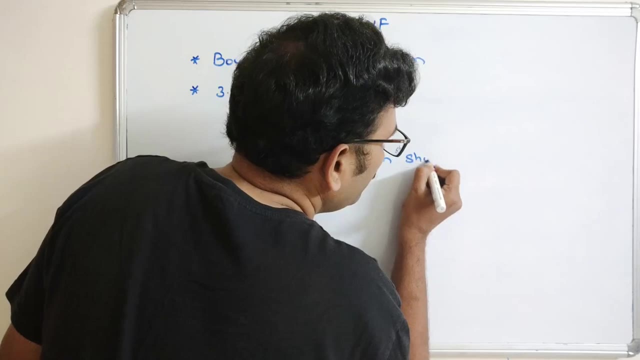 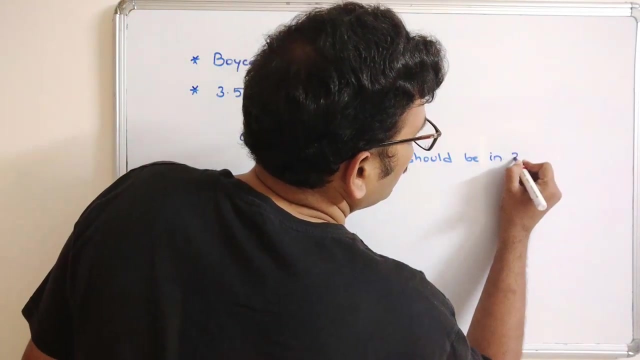 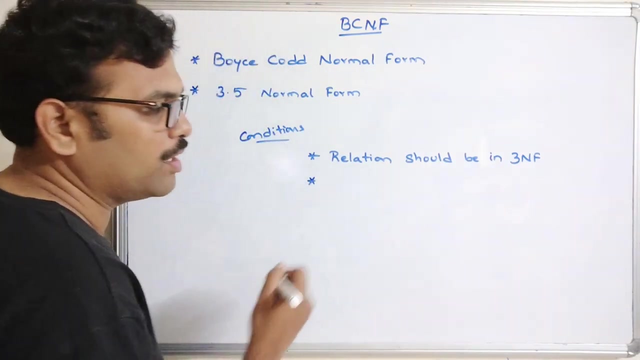 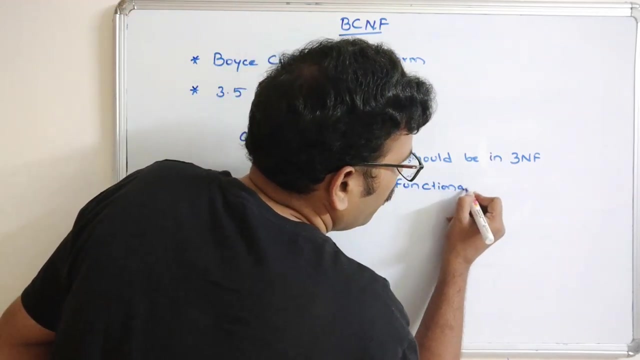 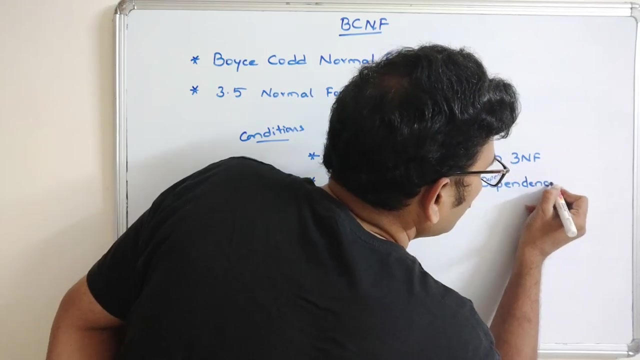 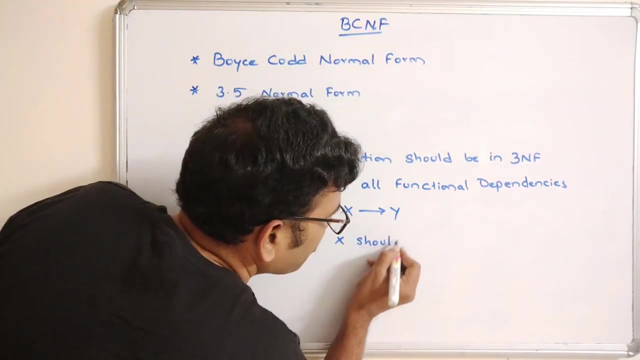 So here are the conditions need to be satisfied. The first one relation should be in 3NF. The relation should be in 3NF, And the second one, the second one, for all functional dependencies. for all functional dependencies, it will be: x tends to y, So x should be primary, key, So x should be primary. 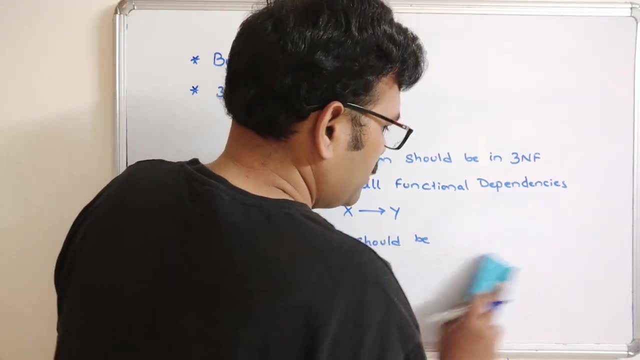 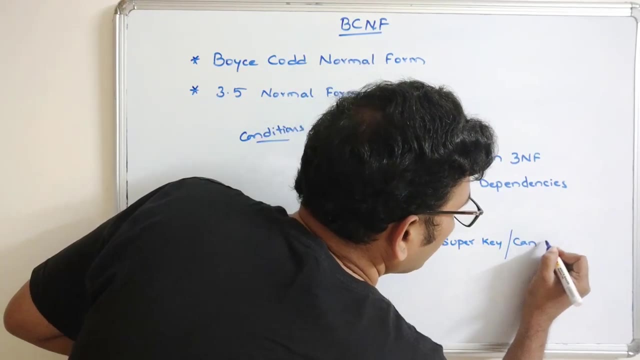 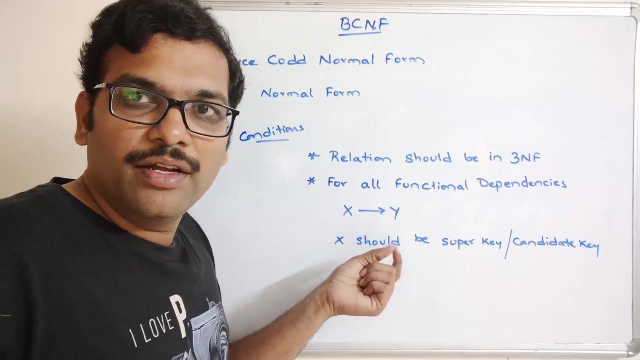 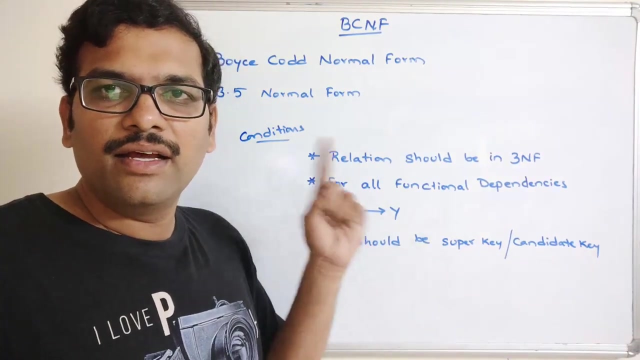 or not super key, Super key or candidate key, Candid key. So for all the functional dependencies let it be x tends to y. So it should satisfy that x should be either super key or a candidate key. Then we can say the relation is in BCNF, right. So first the relation should be in: 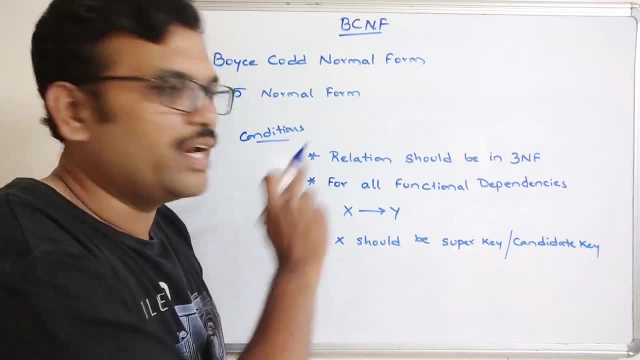 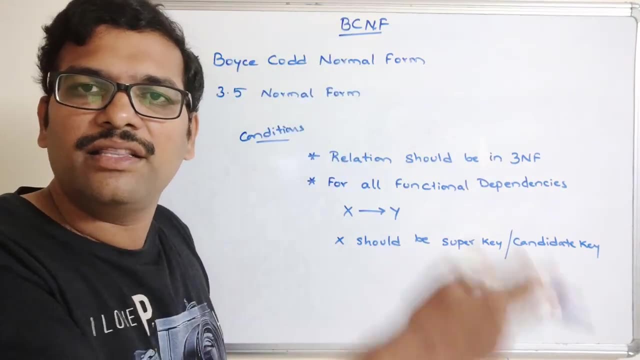 NF. So then only, we have to go with the second condition: If the relation is in 3 NF, we can go with this one. If any relation is in BC NF, we can say the relation is in 3 NF. But if any relation 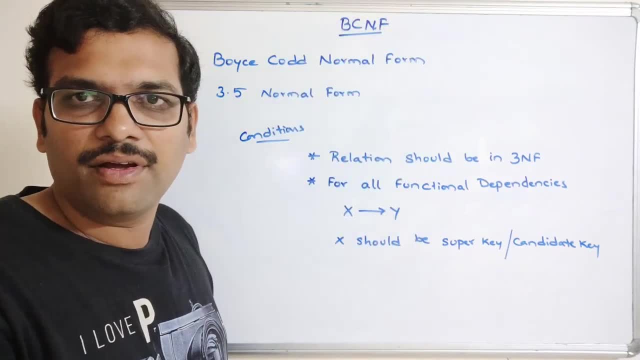 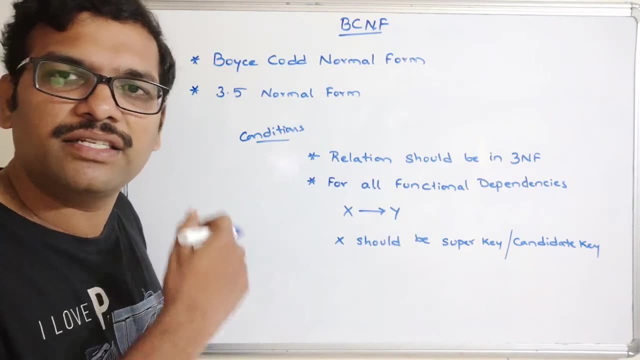 is in 3 NF. we cannot say that relation is in BC NF. So this is a stronger than the 3 NF. So BC NF is a stronger than the 3 NF and still it will reduce some sort of anomalies and redundancies. 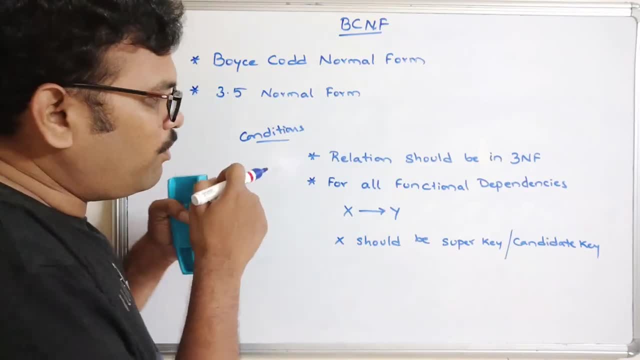 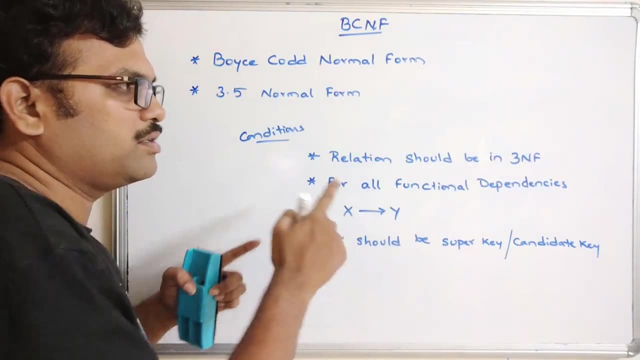 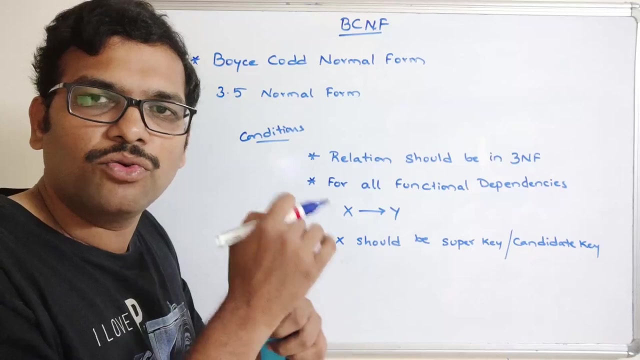 which are available in the 3 NF. So first you have to know what is the 3 NF and how this relation satisfies the 3 NF. So I will completely give the link of playlist in the description section. Go through that So get an idea about functional dependencies. what is a functional? 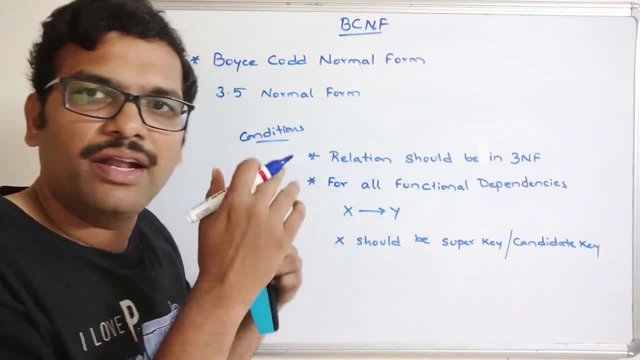 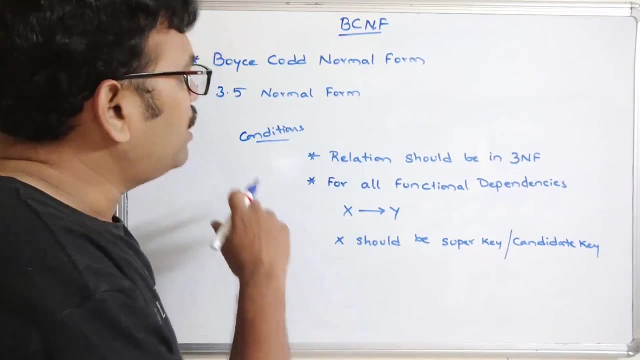 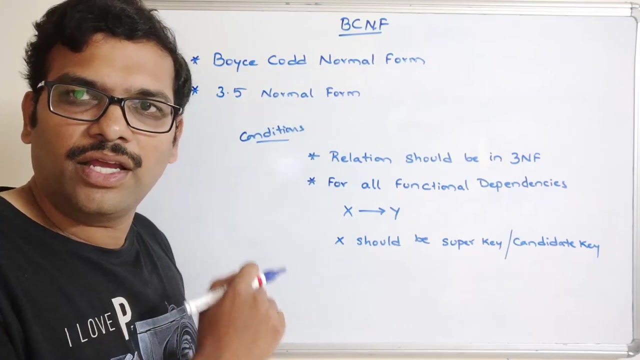 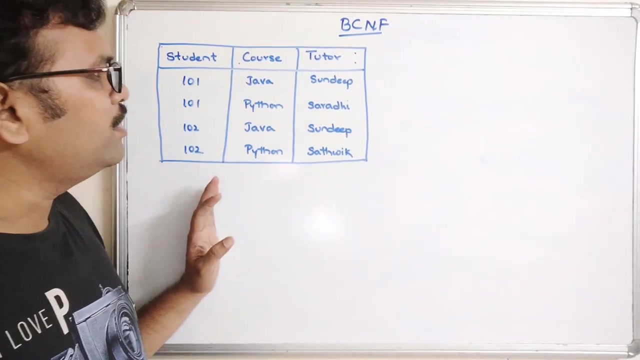 dependency and how the relation should be in 3 NF and everything, and then you will understand this session Very clearly. So let us take one example and I will show you how we have to convert the 3 NF to the BC NF, How we can achieve the BC NF. So let us take this example, consider this relation. 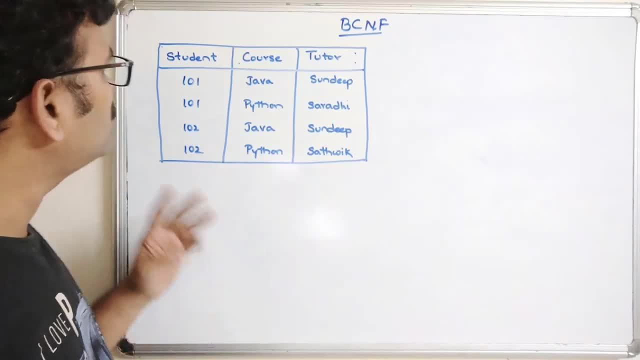 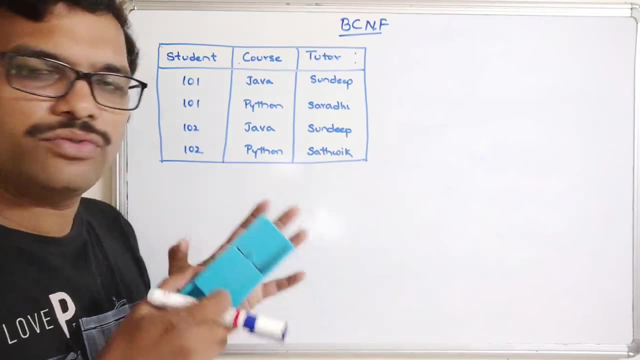 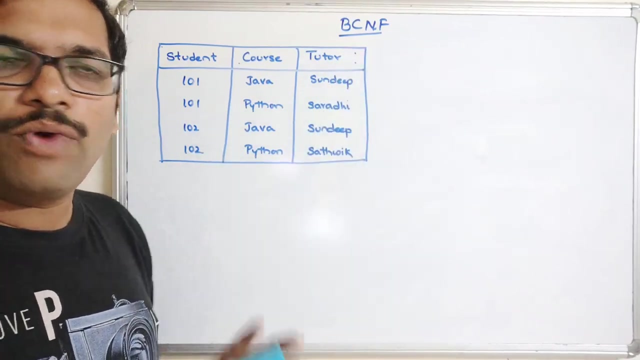 So this relation consists of three attributes, that is, a student course and a tutor. So here we are having a different relation. So first we have, we have to check whether this relation is in 3 NF. So if it is in 3 NF, then only we have to proceed with the BC NF. So what is the 3 NF? So there should not be. 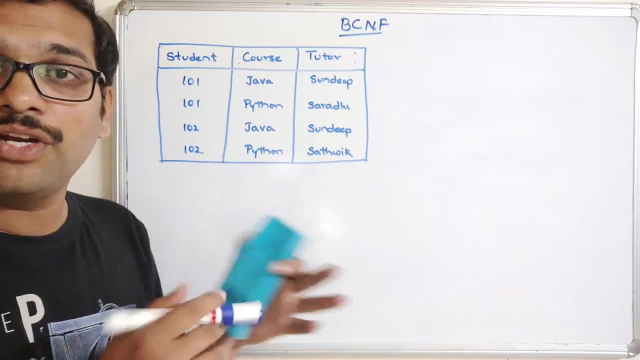 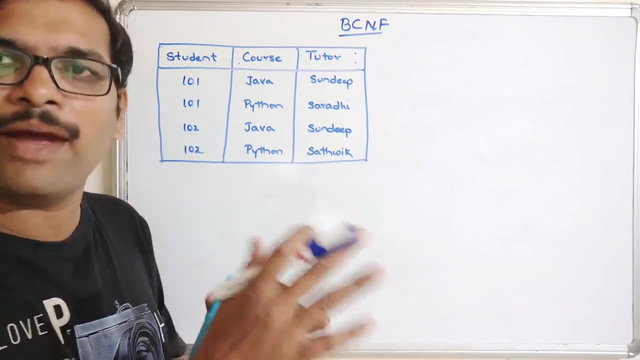 transitive dependencies for the non-prime attributes. So first we need to find the non-prime attributes for this particular relation, and in order to find the non-prime attributes, we have to find the prime attributes. In order to find the prime attributes, we have to find the candidate keys of this relation. 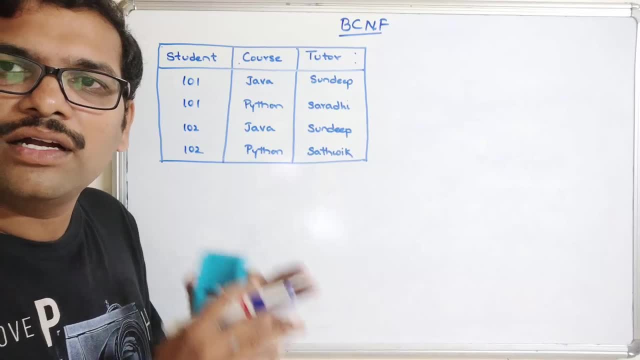 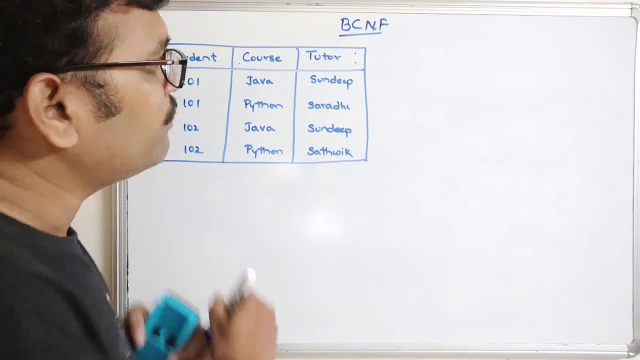 So for finding the candidates keys, first we have to write down the functional dependencies, because even though if we want to check for BC NF, we need to know the functional dependencies. So first let us see the functional dependencies, Let us write down all the possibility, possible dependencies and we will. 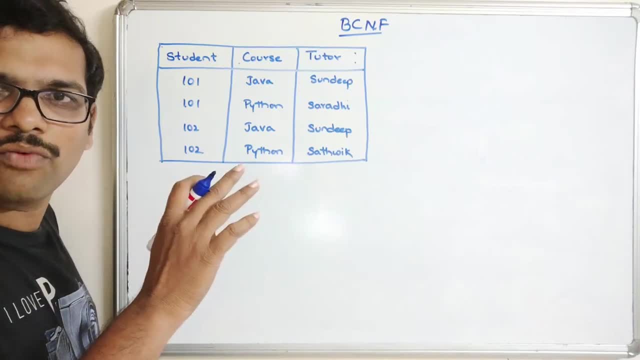 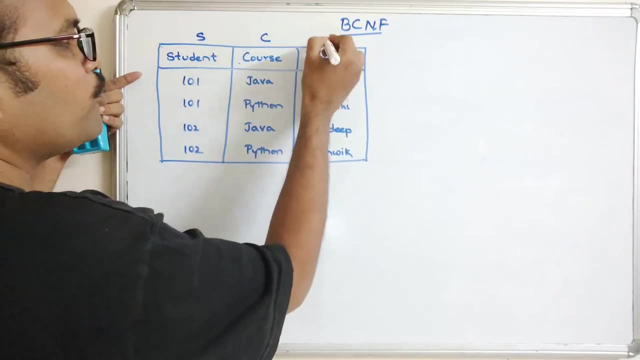 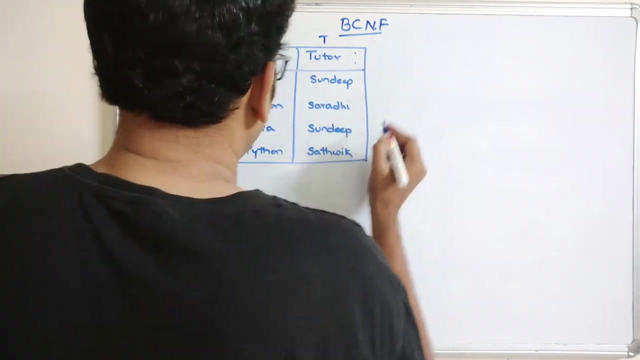 check whether which are the valid functional dependencies and which are not a valid functional dependencies. So I will represent this student as yes, course as C and tutor as T Right? So first let us write down the functional dependencies. So one possibility: yes. 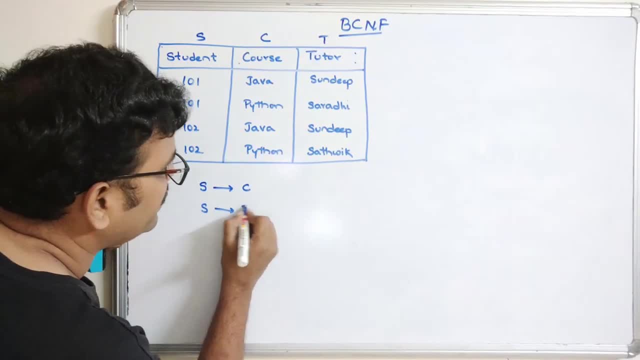 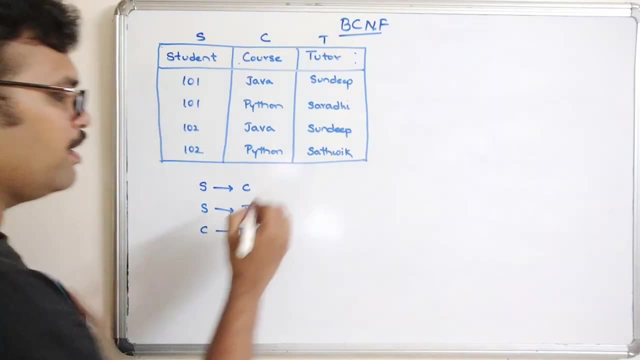 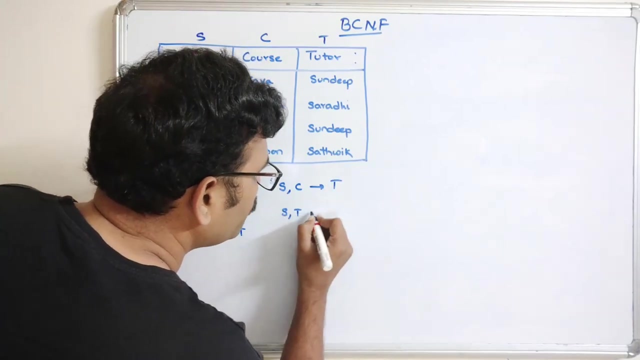 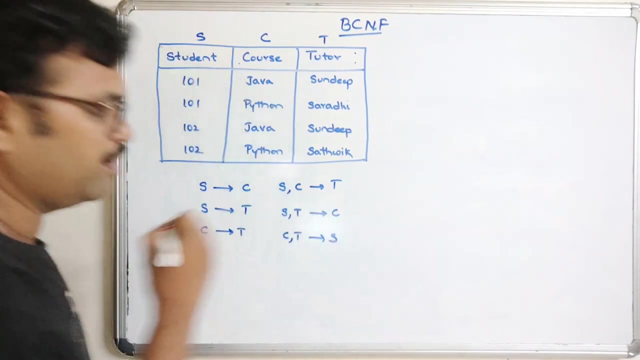 tends to C, yes, tends to T. That means student course, student tutor and also course tutor. And one more one: yes, student comma, course tends to tutor, student comma, tutor gives the course and course and tutor gives the student. So these are the possibilities. 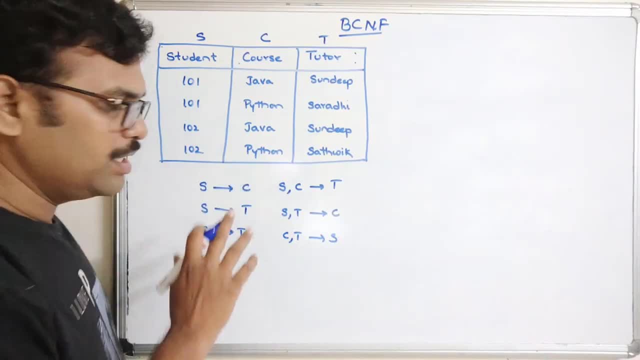 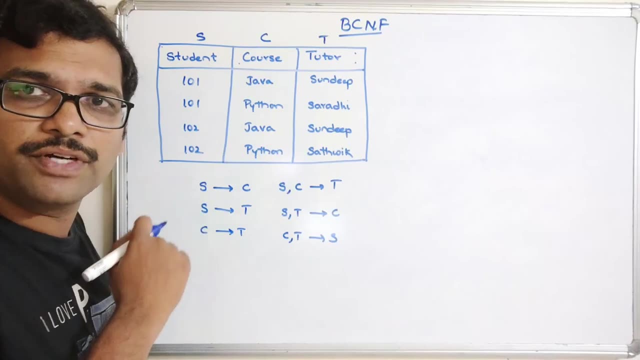 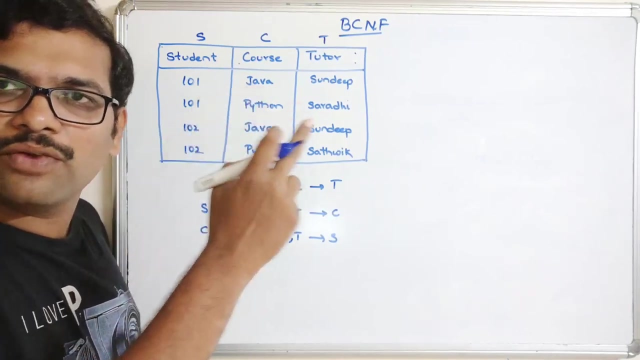 First we will check whether which are the valid functional dependencies. So these are the possible functional dependencies. First, coming to the student. to course, According to our definition of functional dependency, consider two random tuples and if there is a common x value, the corresponding y values should also be same. Then only we can say: 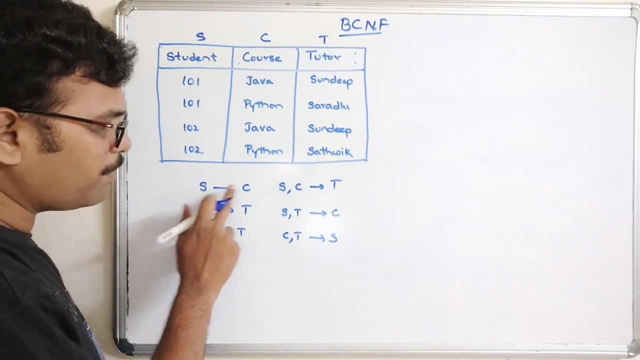 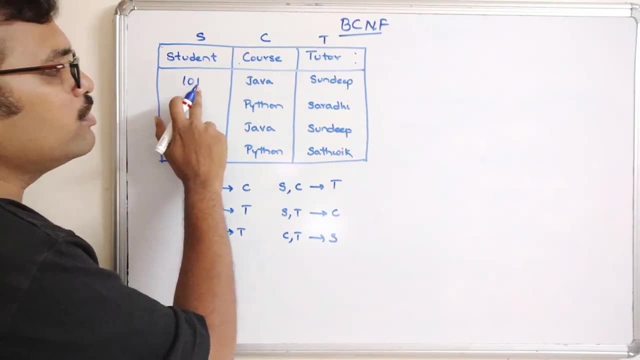 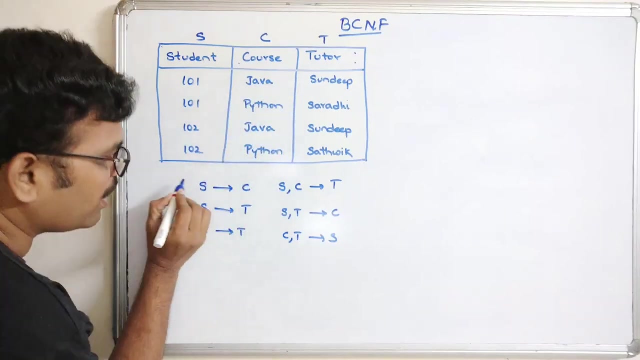 it as a functional dependency. So student can determine the course. So student can determine the course. Consider the first one and second one, 101. It gives a Java and here 101 gives a Python. So one student. we are having a multiple courses so we cannot consider this one. So x value is same. 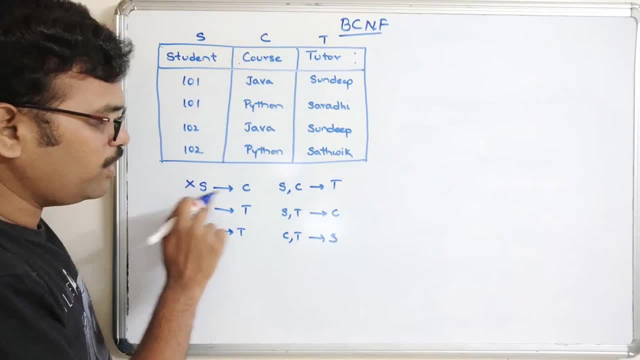 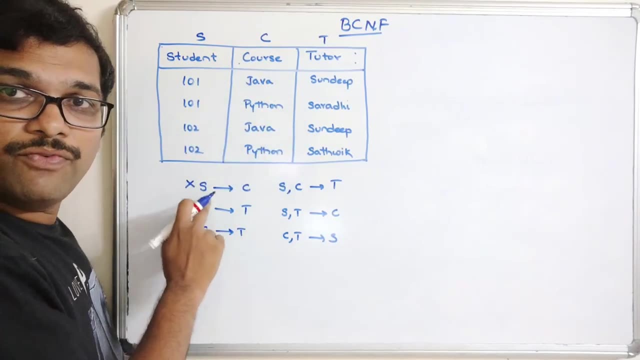 but y value is different. x value is same. This is x value, This is y value. The x value is the same for two tuples but we are having a different y values. So this is not a valid functional dependency. Coming to the student tutor: here also we can see the x values. student. 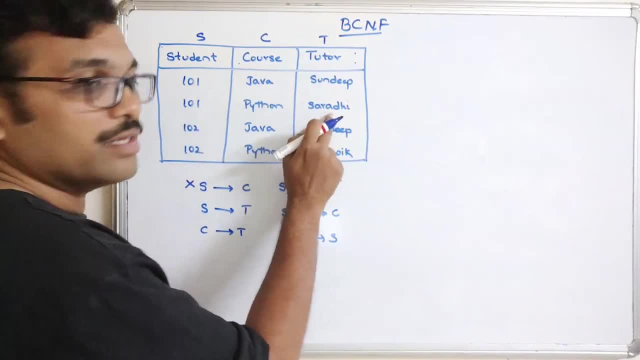 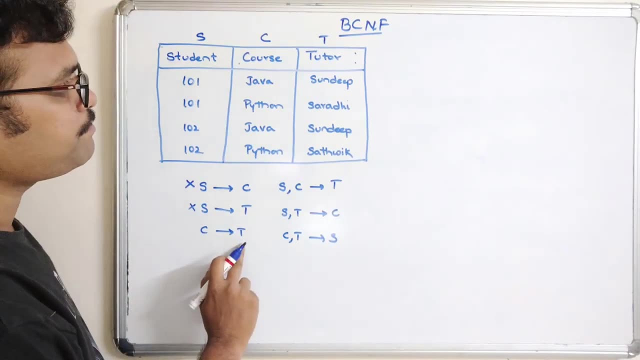 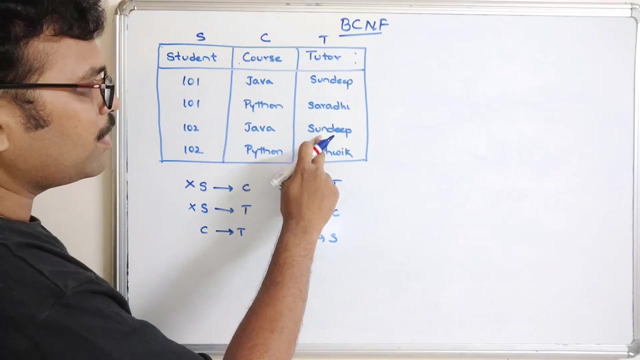 and y value: total 101 Sandeep and 101 Sarve. So this is also not possible. This is also not possible. so course tends to tutor. so Java Sandeep, Java Sandeep. yes, but what about the thing Python Sarathy and Python Sarathy. so this is also not. 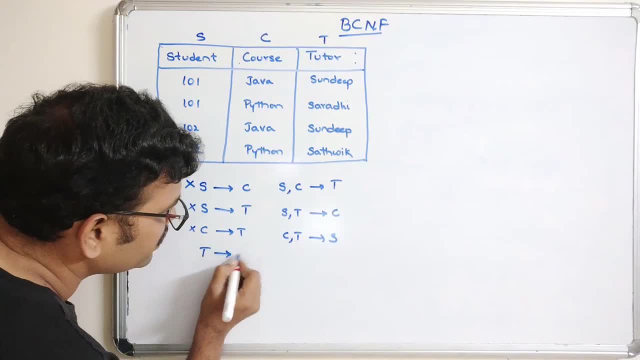 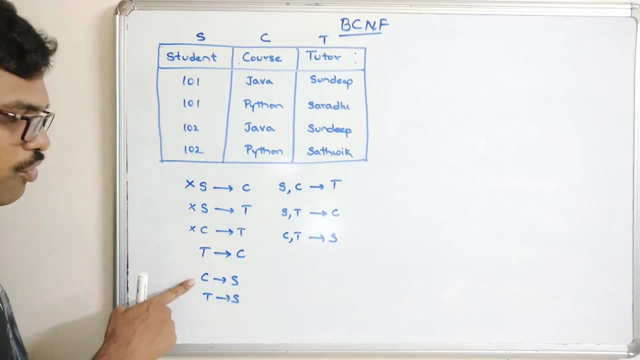 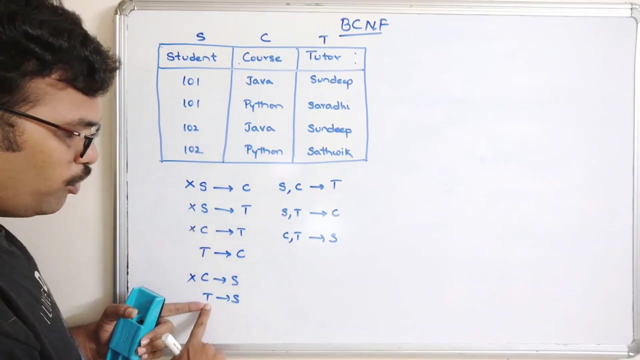 possible. okay, let us assume with the T tends to C. okay, so here also you can see: C tends to yes, T tends to yes. so if you know course, we can get a student details. so for Java 101, Java 102, this is not possible. tutor tends to student. tutor. 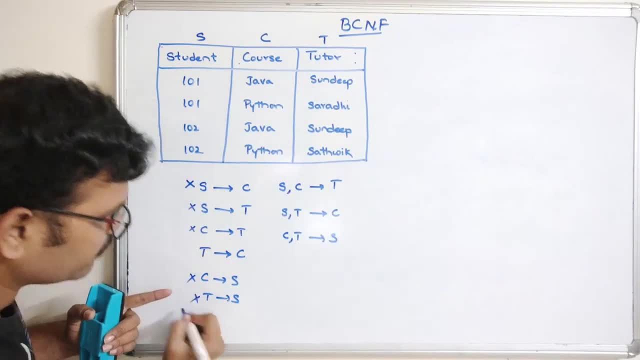 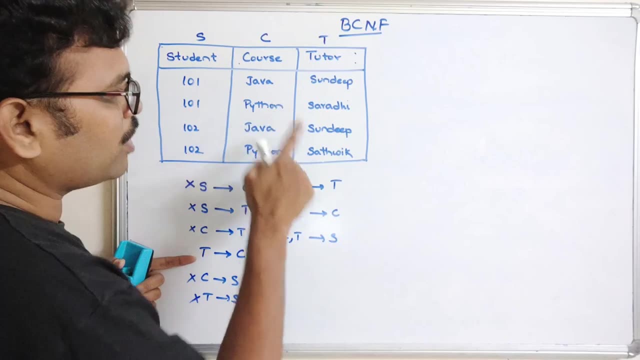 Sandeep 101 to Sandeep 102 is also not possible, and tutor to course. so Sandeep Java, Sandeep Java, Sarathy Python and Sarathy Python. so there is different X values but the same Y values. that's not no problem. okay for different X. 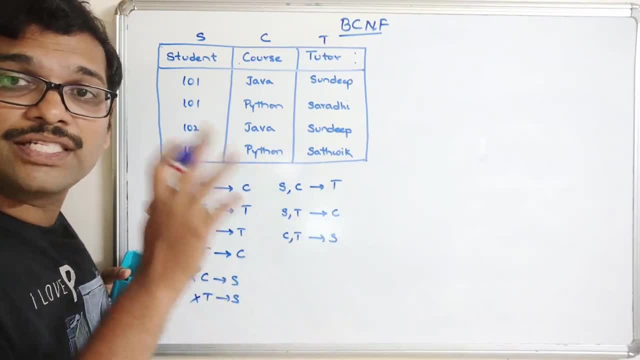 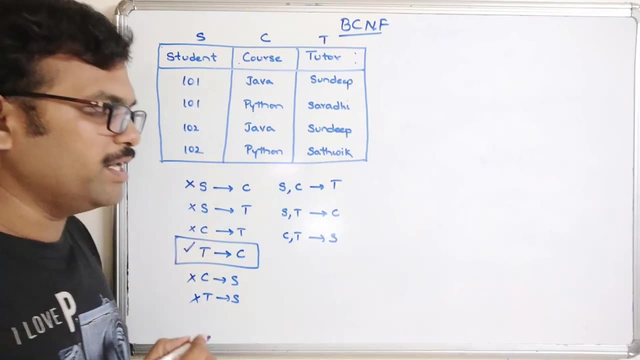 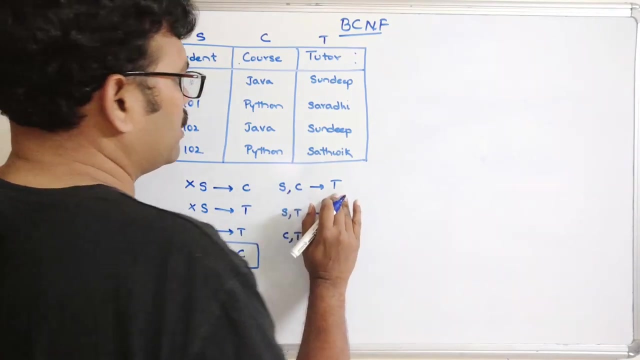 values, different X values, we can get the same Y values, but for the same X values we need to get a same Y value. so this is possible. this is the val will lead. function dependence is the valid functional dependence. so coming to here students in post, give a tutor: student N course 101 Java. so if there any repetition for 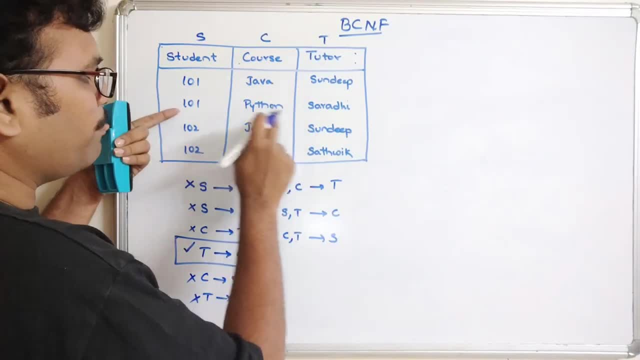 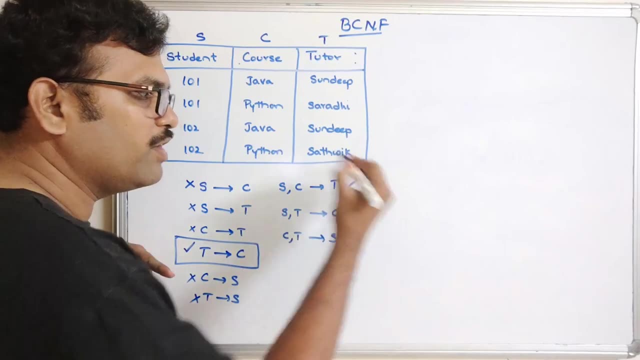 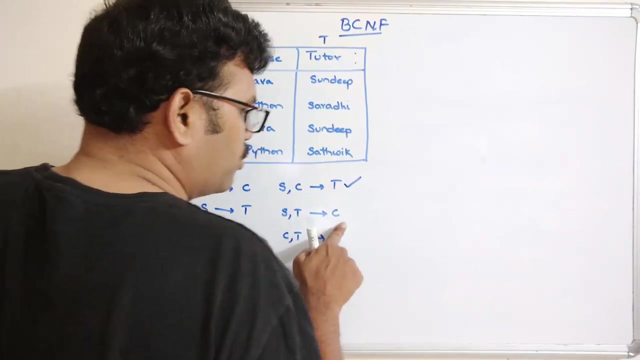 this one one or for Java, no, so one or two. 401 Python: there is no reputation 102, Java, no reputation 102. is there no reputation on x value, so obviously really functionally dependent. next estayn's Students to: T: gives a C, That means a student along with the tutor, gives a course Student. 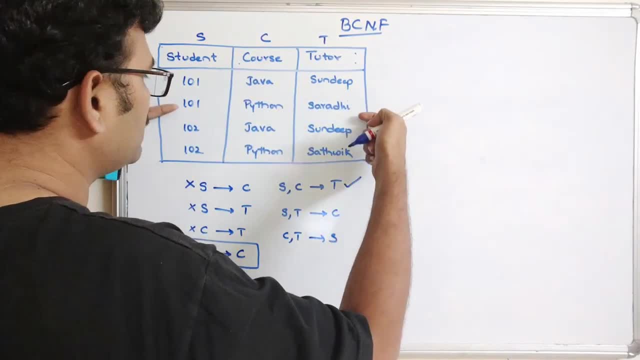 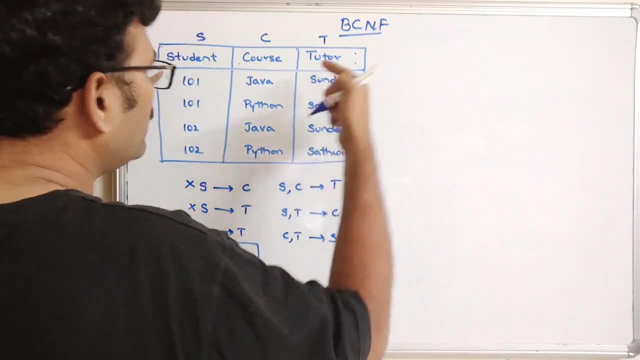 along with the tutor. 101 Sandeep. Is there any 101 Sandeep Here? 102 Sandeep, So that's different. 101 Sarabhi, So there is here. 101 Sandeep- This is a different, So there is. 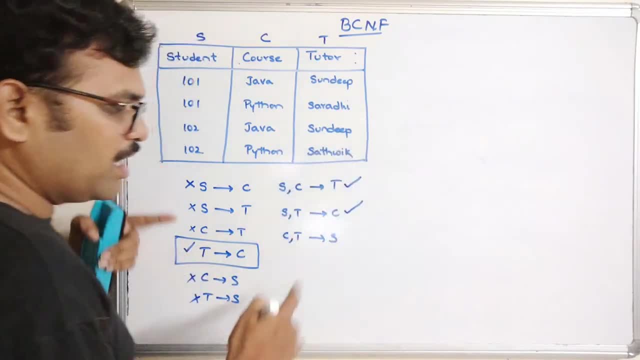 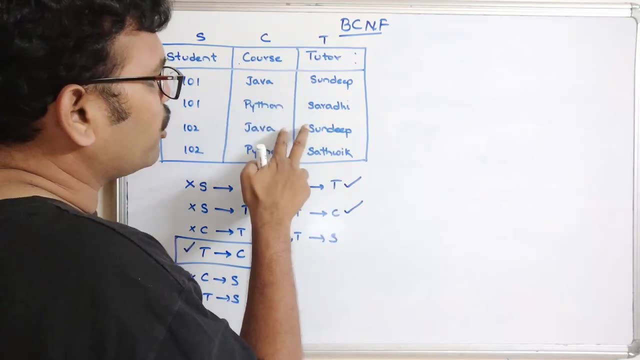 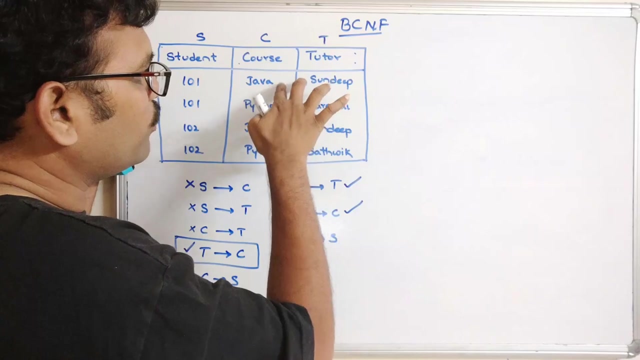 no duplicates, So this is also possible. Coming to the course and tutor gives the student Course and tutor gives the student So course. and tutor Java Sandeep- Here also Java Sandeep, OK So course. and tutor Java Sandeep and Java Sandeep. Both we are having duplicates. 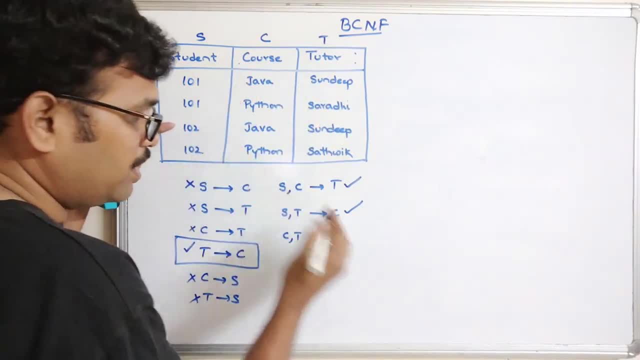 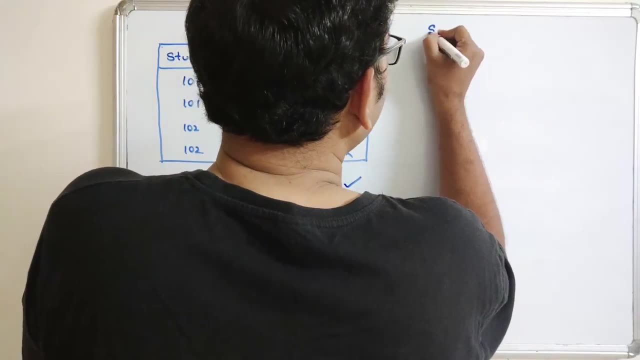 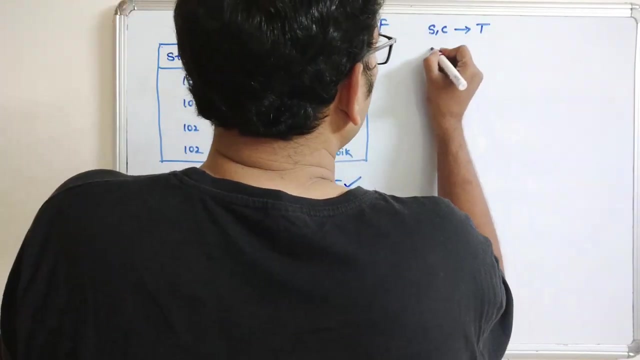 But here y values are 101 and 102.. Both are different, So this doesn't form the functional dependence. So here some valid functional dependencies are. So S comma C: That means a student along with the course can determine the tutor And a student along with the tutor. 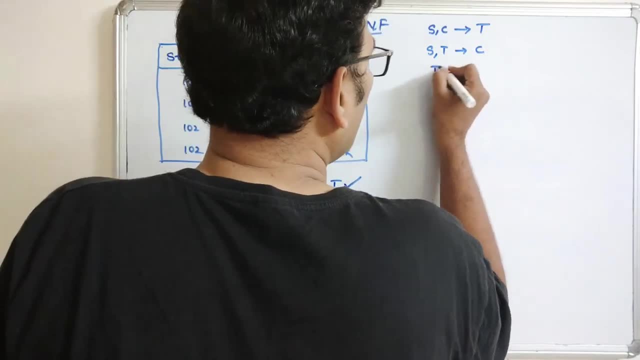 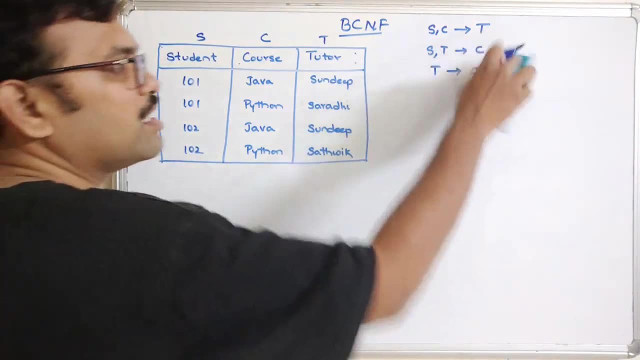 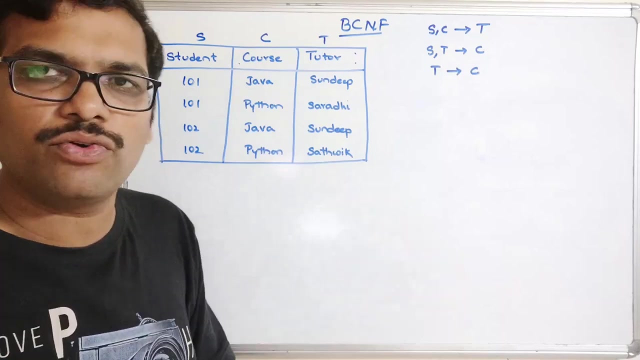 can determine the course And a tutor alone can determine the course. so these are the a few functional dependencies we can. we can say that these are the functional dependencies for this particular relation, right? so once you just practice. so write down all the possibilities and check out that one, so you'll get these three as a 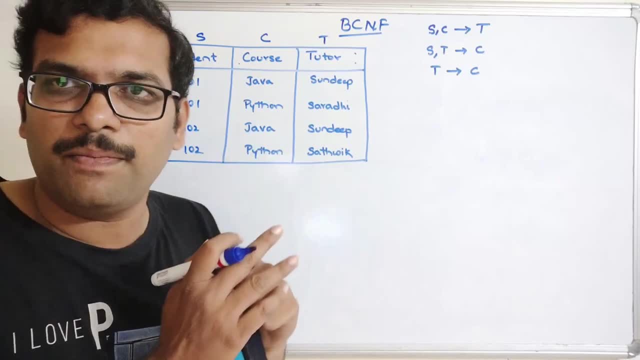 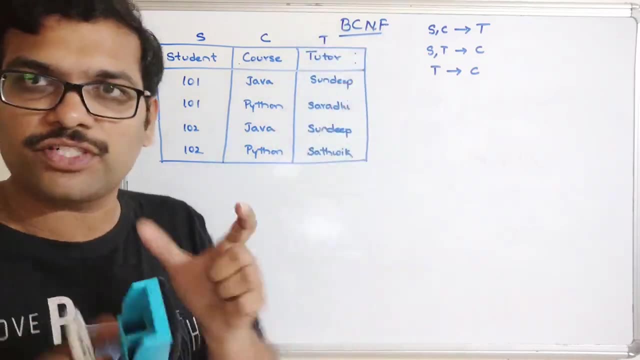 functional dependencies. so the first step is: we got the functional dependencies. the next one: we have to check whether the relation is in 3nf or not. because for checking for bcnf first we need to check whether the relation is in 3nf or not. then only we can go with the bcnf. so what is the 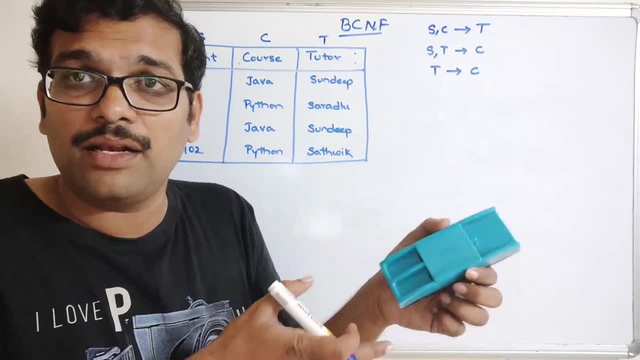 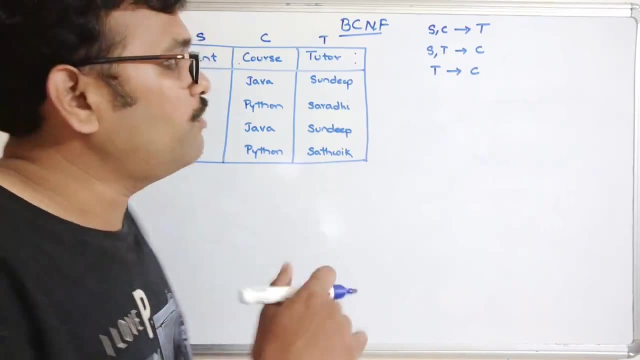 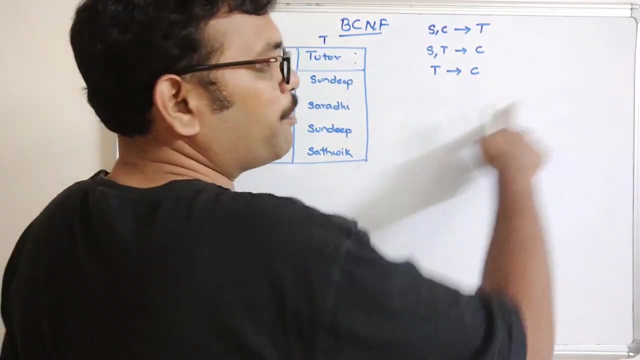 3nf. so if for a functional dependency, that i mean for all the non-prime attributes there should not be, there is a transitivity functional dependency. so for that we have to find the candidate keys. what are the candidate keys? so here, in order to find the candidate keys, write down the procedure. 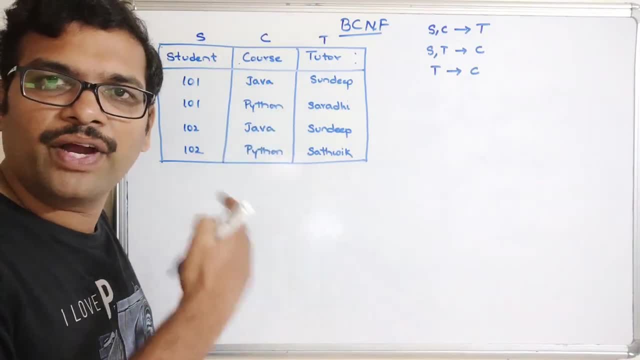 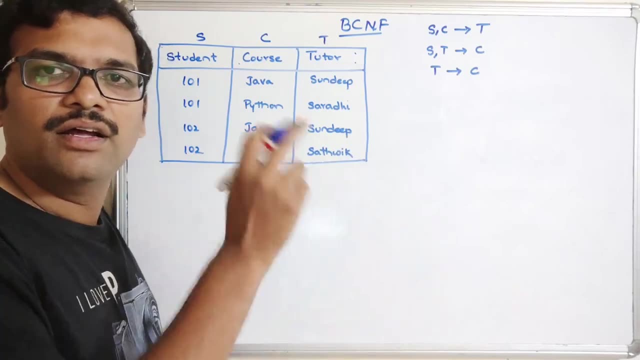 in the previous session we have solved many problems to finding the super keys and the candidate keys, so i will post the link of complete playlist in the description. in that playlist you can find the video and just visit that video and you will be understanding this concept right. so 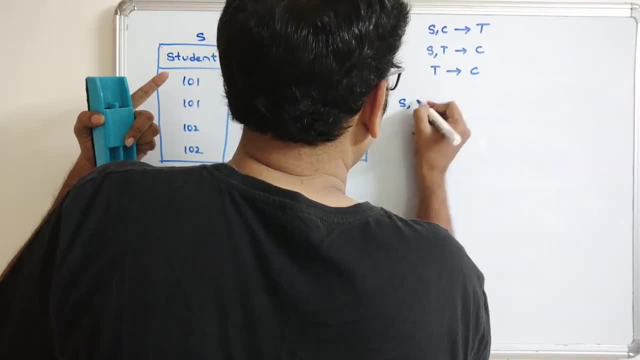 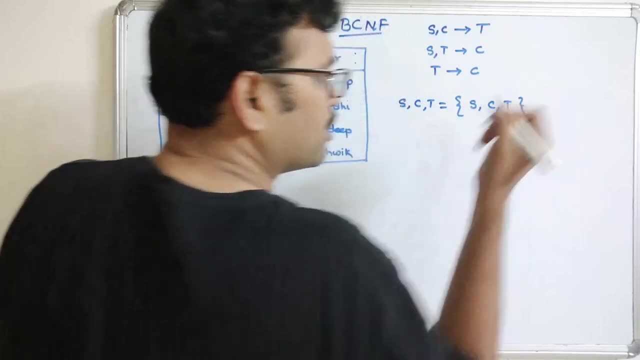 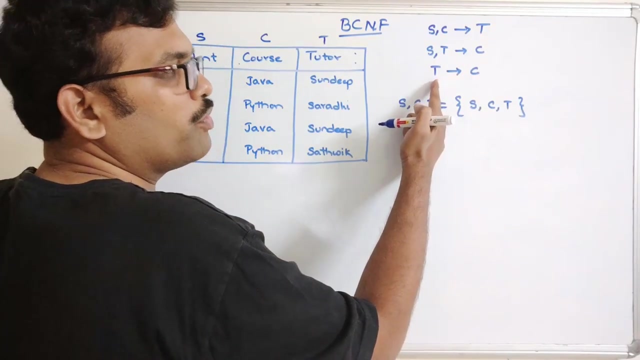 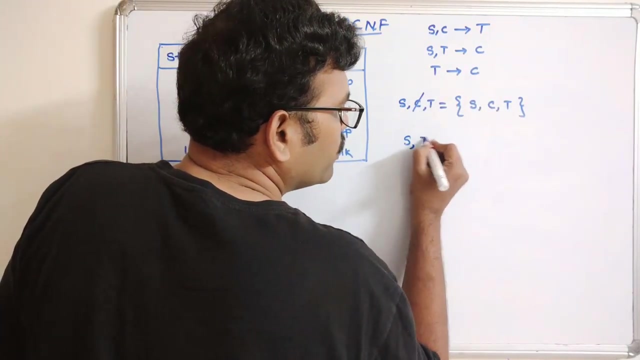 first. so student course tutor will give all the three, so this is a closure. you can say: this is a closure right. so from the functional dependencies, if you know t, that means if you know the tutor, we can get the course. so you can just remove the course so student along with the tutor can. 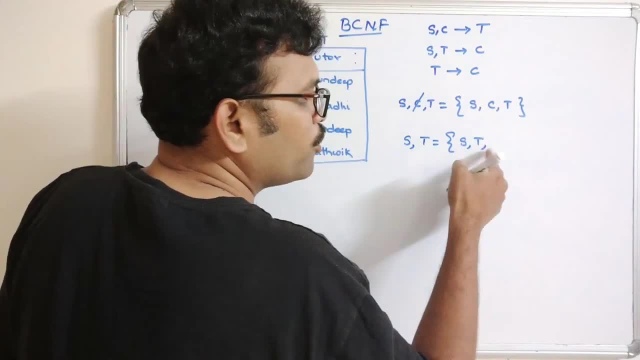 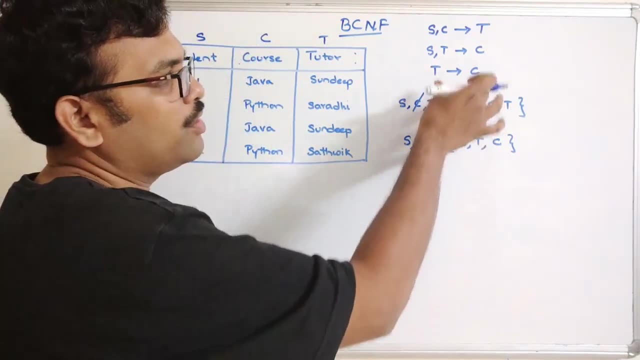 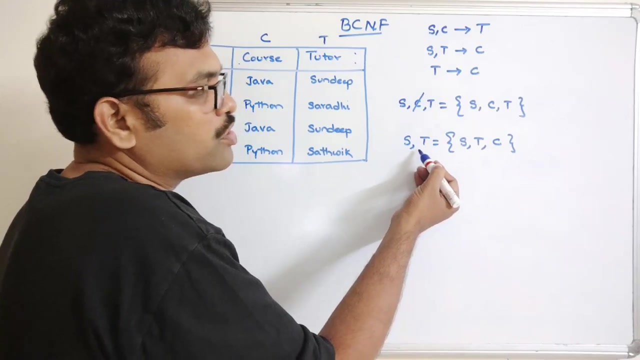 determine student, tutor, and if you know tutor, we can get a course right. so is there any possibility to reduce this one? no, from this functional dependency there is no. if you know student and course, we can get a tutor, but here there is no course, only we are having a student. okay, so this: 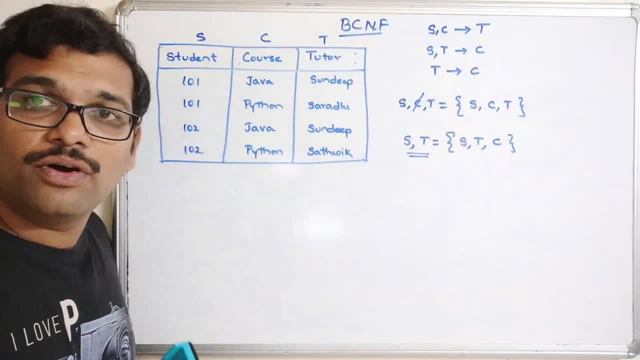 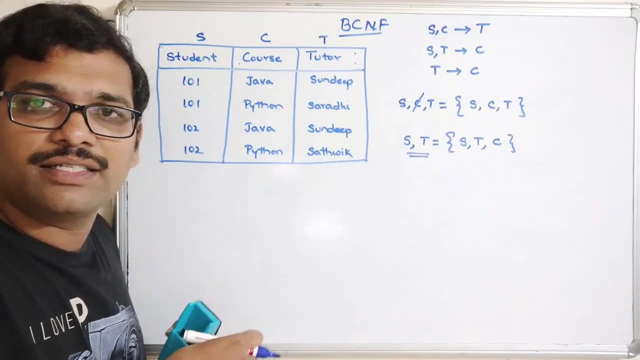 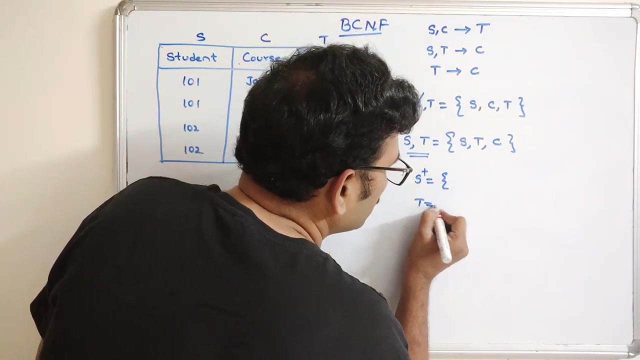 is the one candidate key, so one super key. one super key because, by using the student and tutor, we are getting all the three attributes, but we can't say that this is a candidate key. so we need to check all the possibilities, find out the s closure and the t closure. so for s closure, if you know yes, we can determine yes. 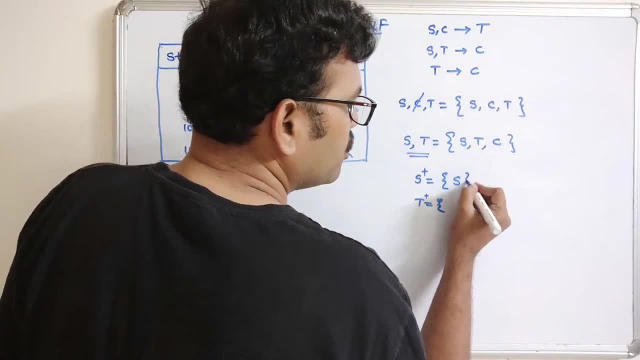 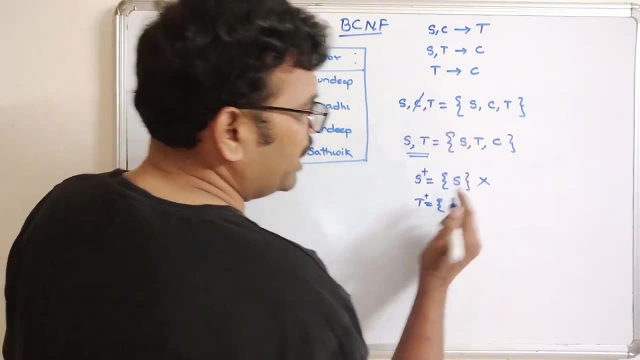 and if you know yes alone, we can't determine any other. so this is not as candidate key. and t plus, t plus. so that means, if you know t, can determine t, if you know t, we can determine c, and if you know both t and c, we can't determine any. 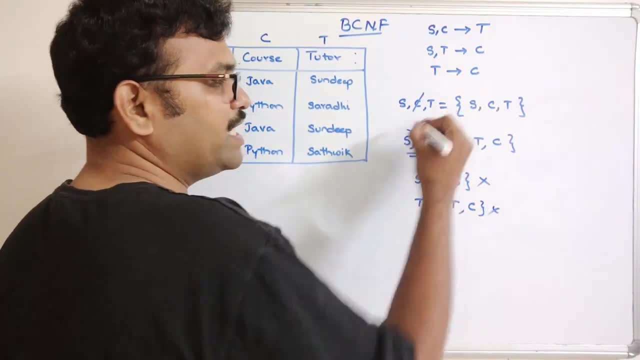 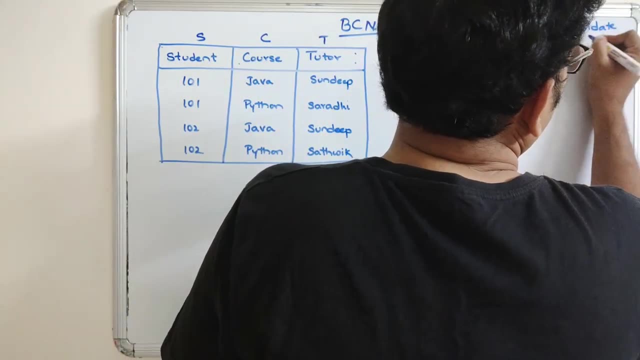 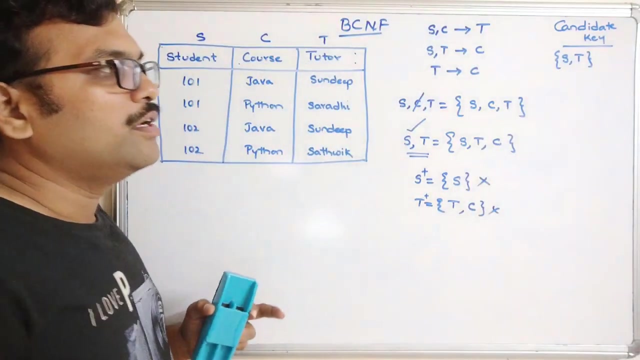 other. so this is also not a super key. so we can determine. we can say that s and t are the candidate key. so here i will write a candidate key. so one candidate key is student and tutor. so we can't say student and tutor are the same candidate keys. so we have to check. 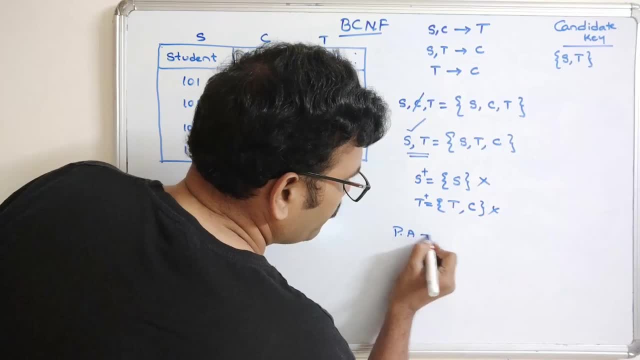 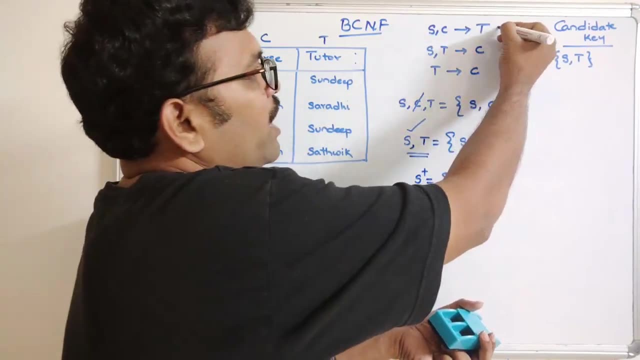 these are the prime attributes. okay, the prime attributes. the prime attributes are s comma t. we need to check whether these prime attributes are on the right hand side of the any relation or not. so we are having one prime attribute as a right hand side of the functional dependency. so replace. 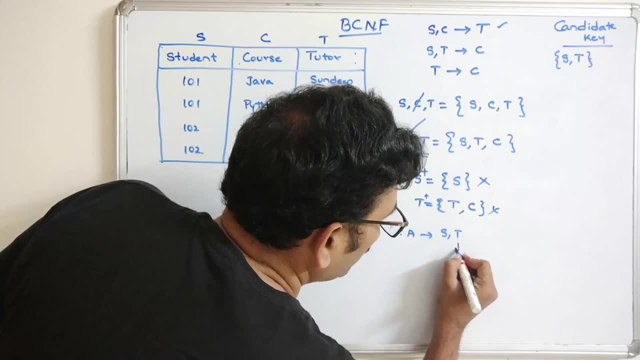 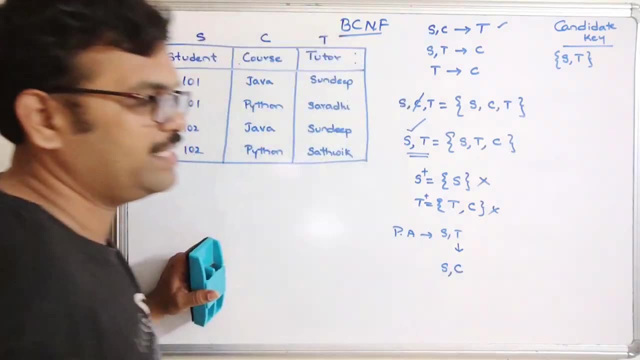 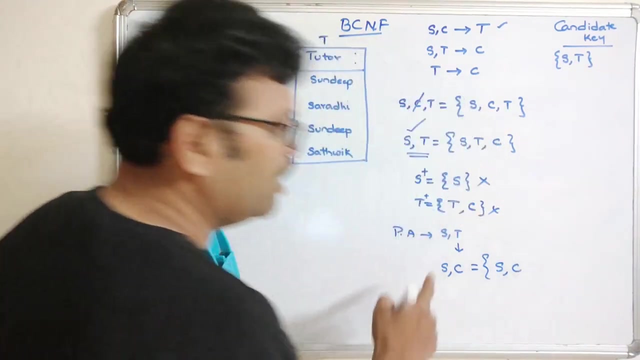 this one with this one, so you can replace this one. so, yes, comma in place of t, we can give s. comma c, which we can. yes, is already there, so we can give c right and again find out the closure, whether we can find out or not. yes, comma c. if you know a student and a course, we can get a. 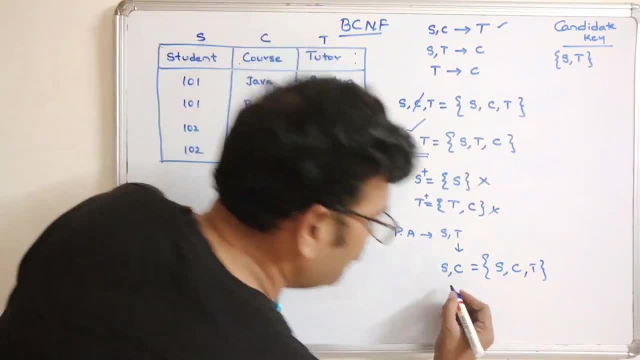 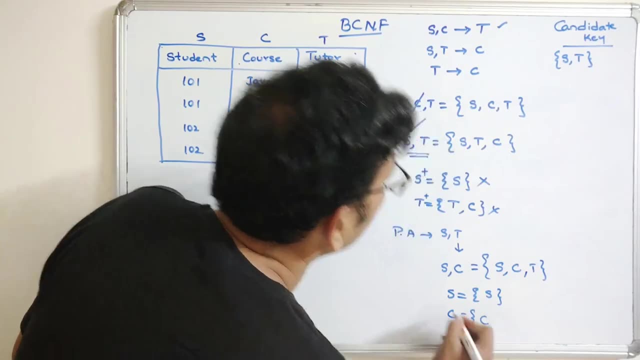 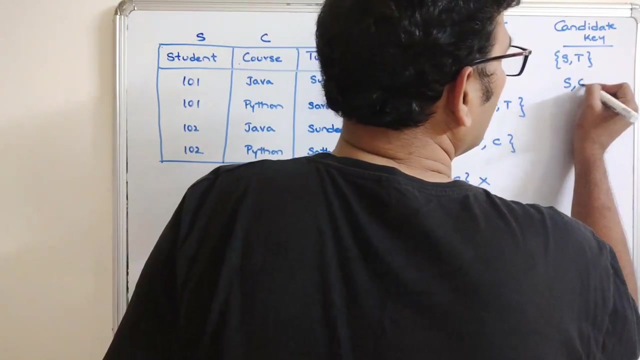 t, so this is a super key. we can say this is a super key and minimize this one. so, yes, so you, by using s, we can get only s. we're using c, we can get a c, and if, by knowing c, only the c can be determined, so this is this, this is not a super key. so yes, comma c: again, it's a candidate key. 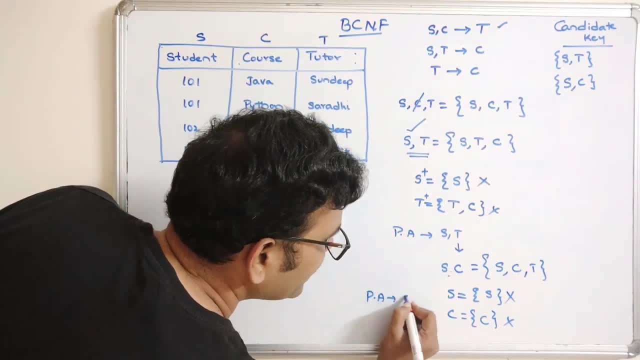 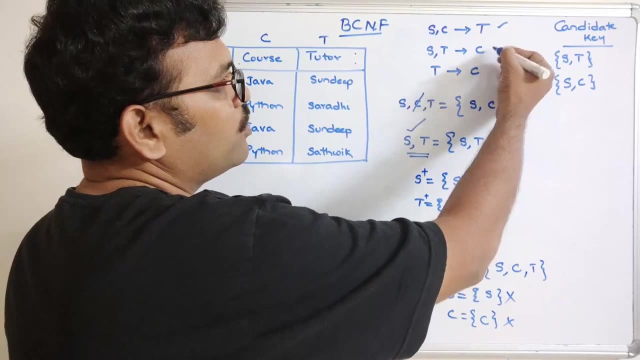 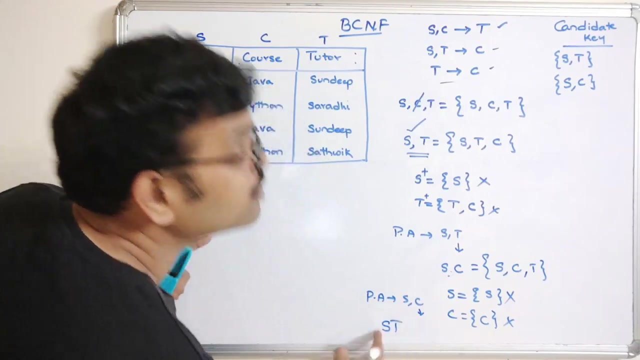 again, find out the prime attributes. the prime attributes are s, comma, c, so find out whether these prime attributes are residing on the right hand side. yes, we are having both the things, so consider any one. so consider the third one. so replace this c with t, so s t. so s? t is already a candidate, key student and a tutor, along with the candidate. 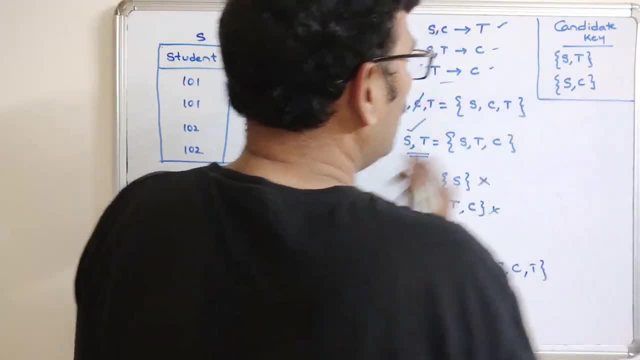 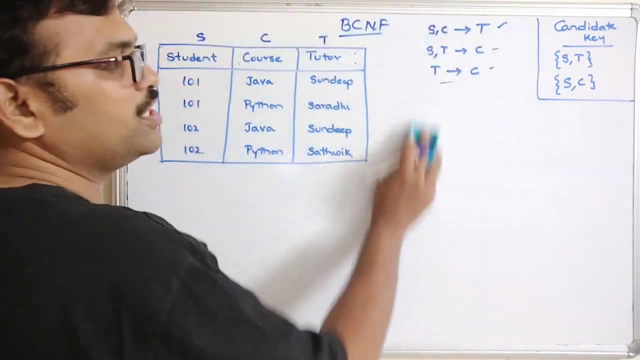 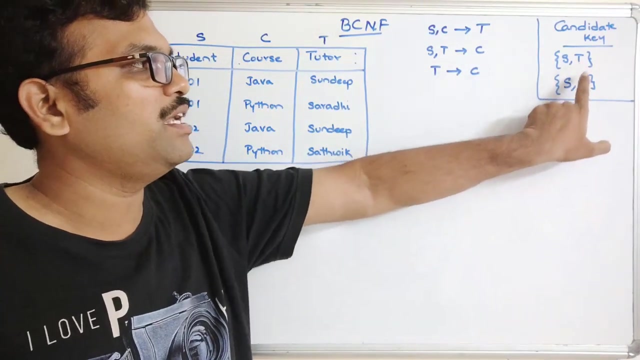 key so you can stop here. so our relation is having a two candidate keys. so just go the procedure by following the previous sessions so you can understand the procedure. so from that procedure, by following that procedure, we have find out the candidate keys are s comma t and s comma c and what we have to check: whether the non-prime attributes what are the non-prime. 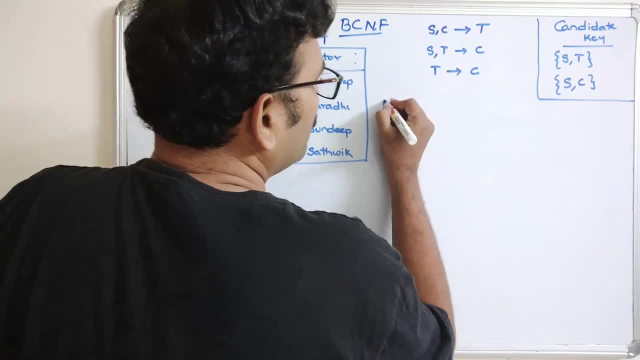 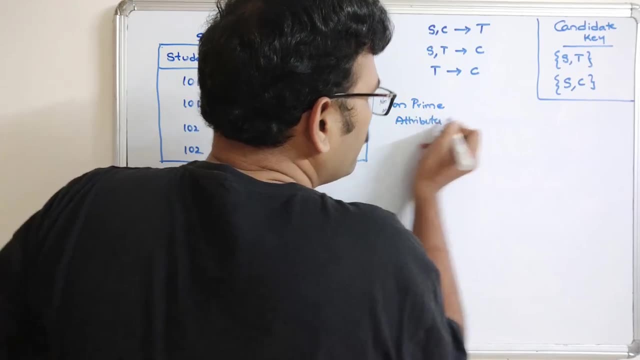 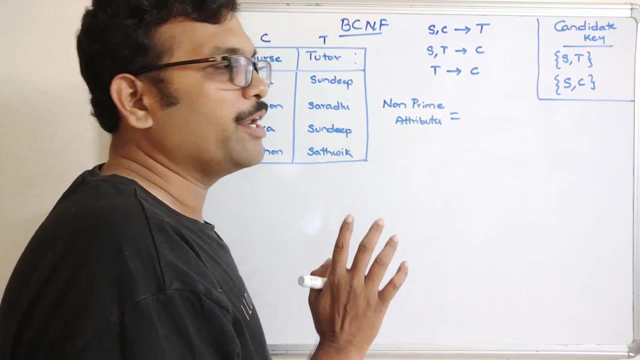 attributes. so i'll write here: so non-prime attributes are the attributes which are not available in the candidate key. so you can see from this one we are getting all the things. there is no prime attributes, non-prime attributes, okay, no non-prime attributes. so obviously there will be no three. three, i mean it follows the. 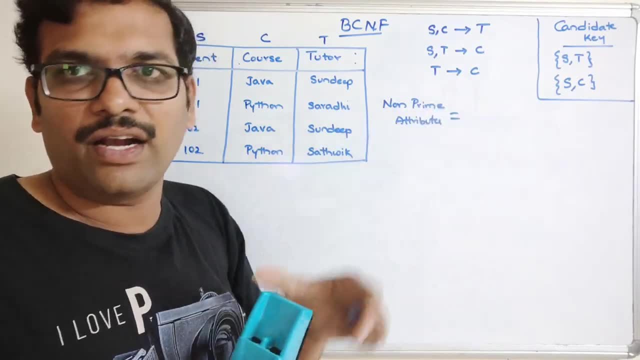 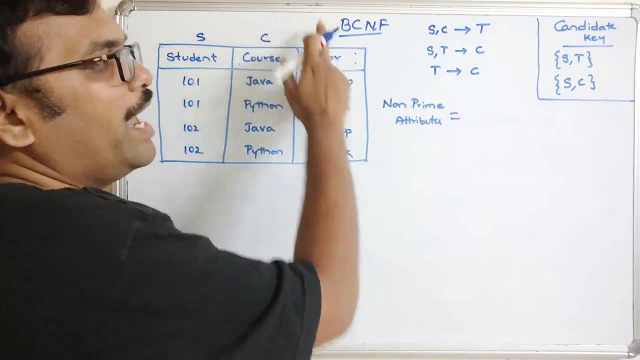 three nf. there is no transitivity dependency for the given relation because we are not having any non-prime attributes. all these are the prime attributes: yes, t and c. we are having the three attributes and all the three are available in the candidate key. so there is no prime non-prime. 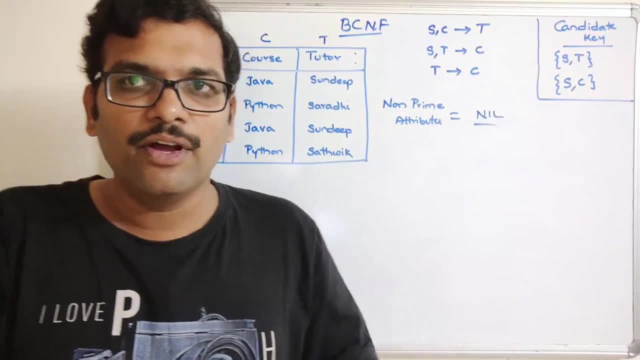 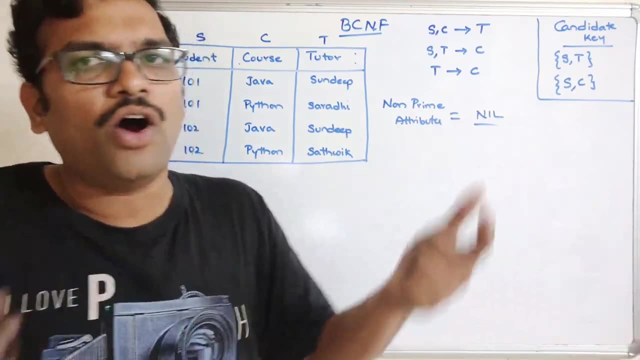 attributes. so in order to check whether the relation is in three nf, we have to check. there should be no transitivity dependency for a non-prime attribute. but here we are not having any non-prime attributes, obviously the relation will be in three nf, so no non-prime attributes. so 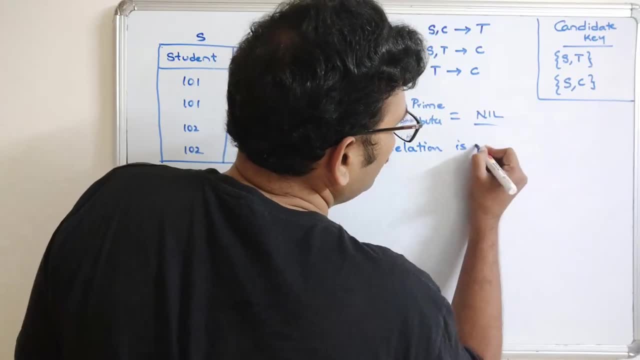 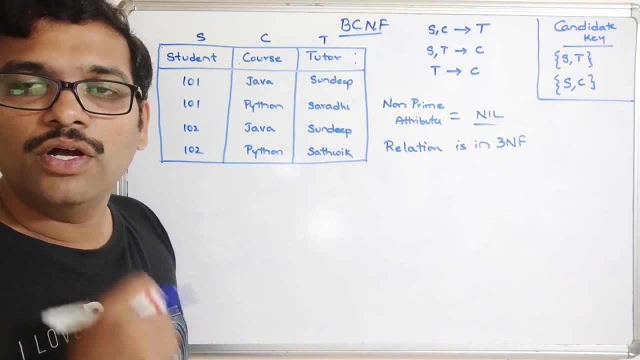 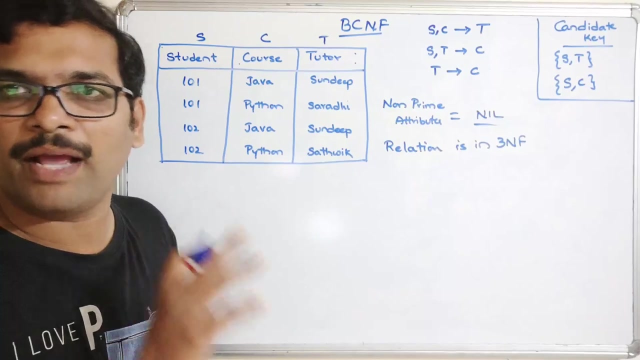 a relation is in three nf. now we have to check for the bcnf, whether it is in bcnf or not. so what we have to do, we have to check whether, if for all the functional dependencies, x should be the super key or a prime or a candidate key. so for this functional dependency, you can see s comma c, which is a candidate. 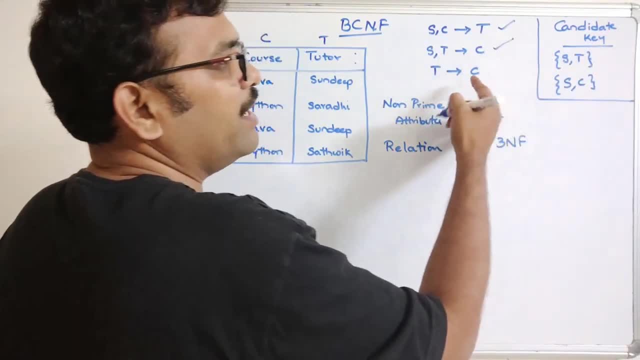 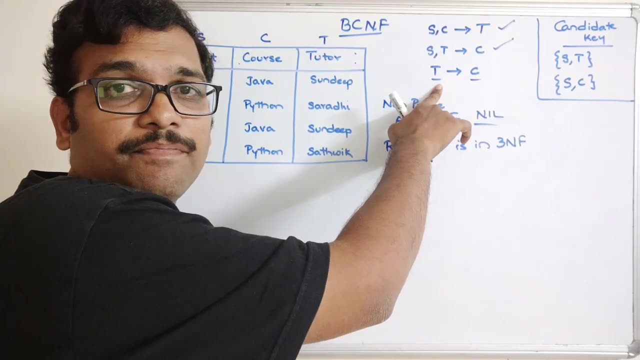 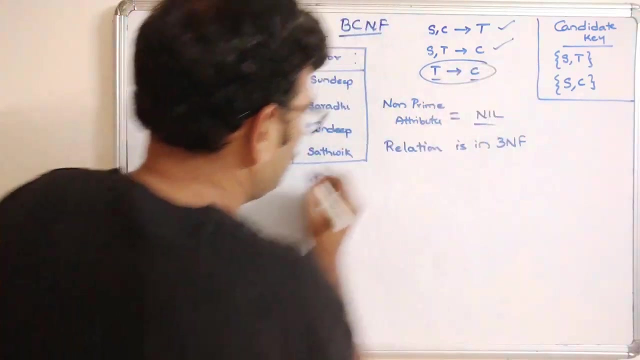 right s comma t, which is a candidate key right and here t tends to c. here it is x and it is y, so x is not a super key or a part of candidate key. oh sorry, it's not a candidate key, not a path. okay, it's not a candidate key, so we have to. so here you can see t tends to c, so t is not a. 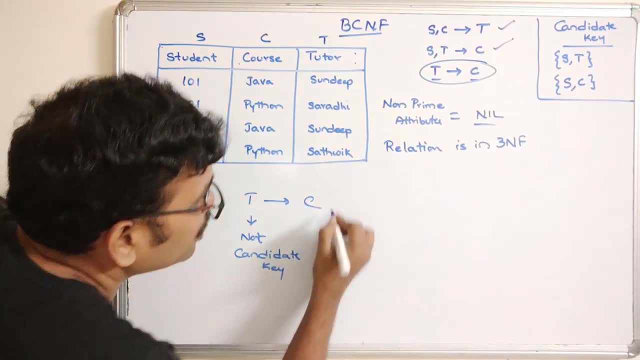 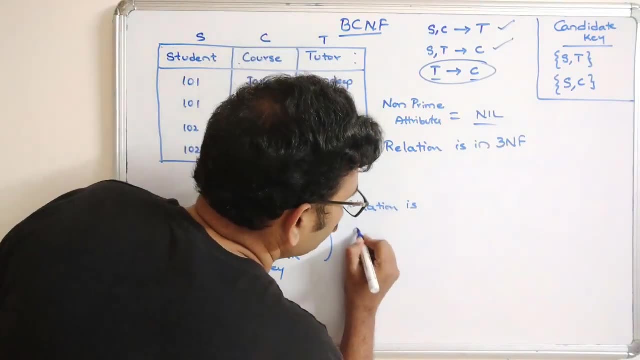 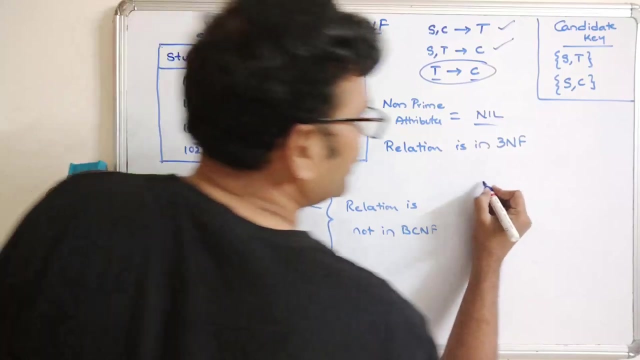 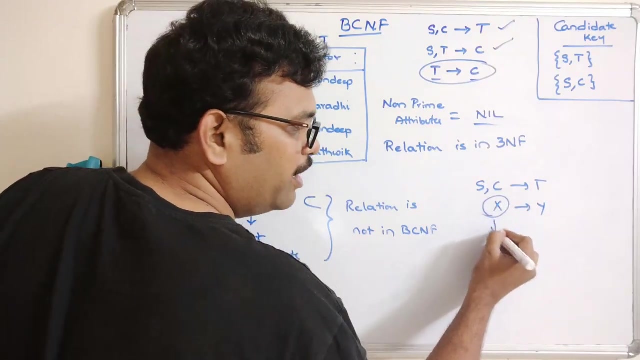 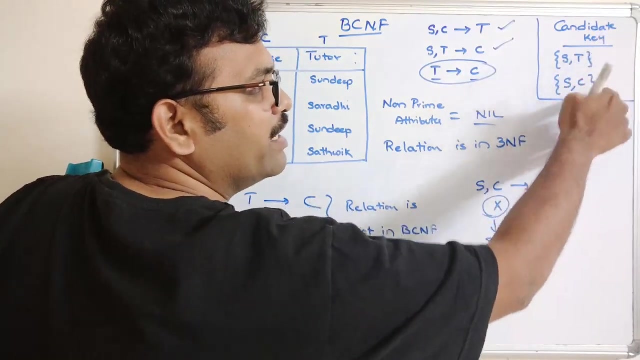 candidate key, candidate key. so relation is not in bcnf. so if, if, for example, for these two things, s comma c tends to t, so here it is x comma y, x tends to y, so x should be a super key or a candidate key. okay, super key or a candidate key. yes, yes, comma c is a candidate key c, so this is a valid. 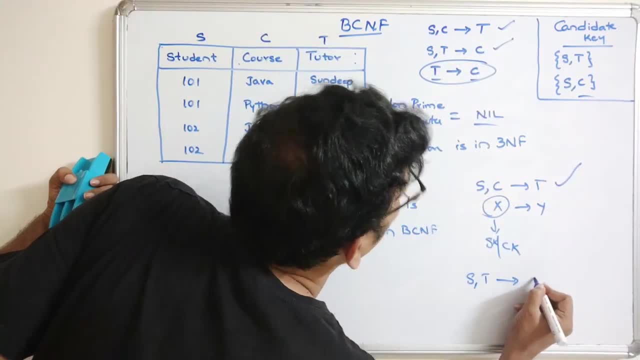 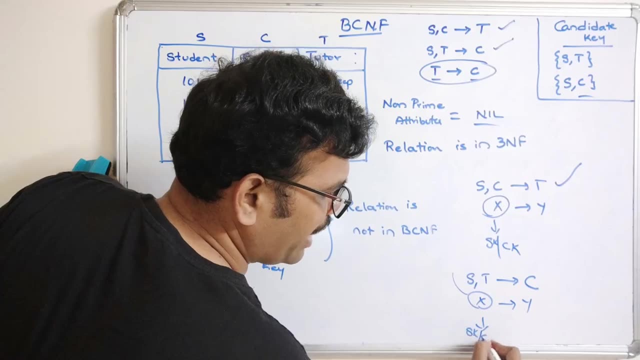 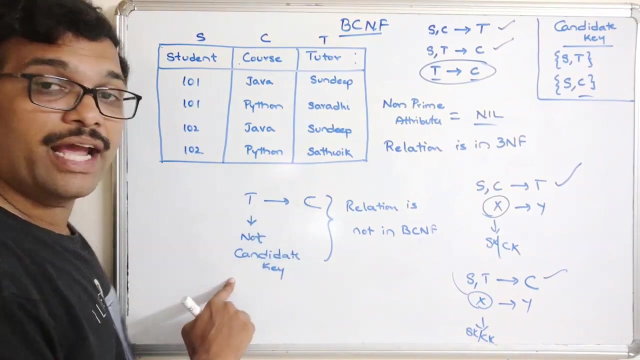 second one: yes, comma t tends to c. so here you can see this is the x and this is y. so x is again it's a super key or candidate key. yes, comma t is a candidate. yes, so, coming to this one, x, comma y and x is not a candidate key. obviously we can say the relation is not in bcnf. so if the 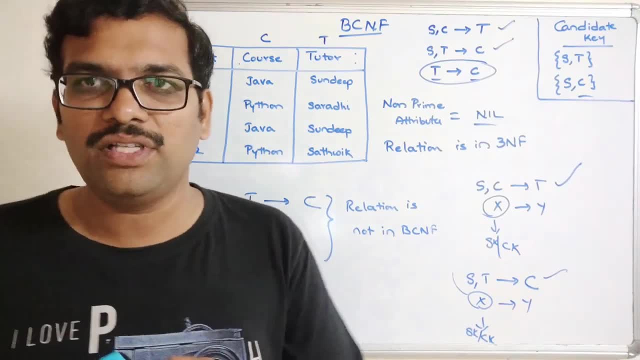 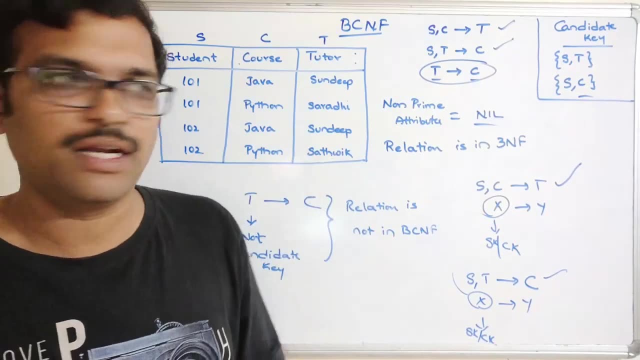 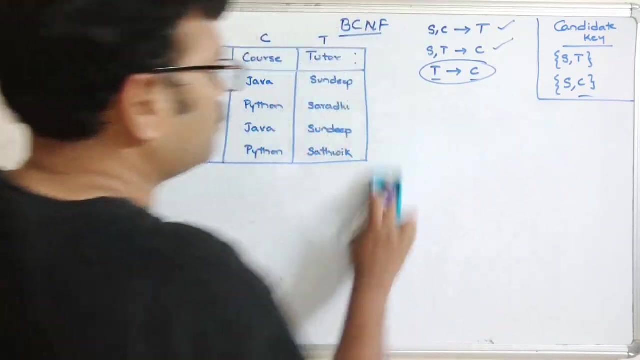 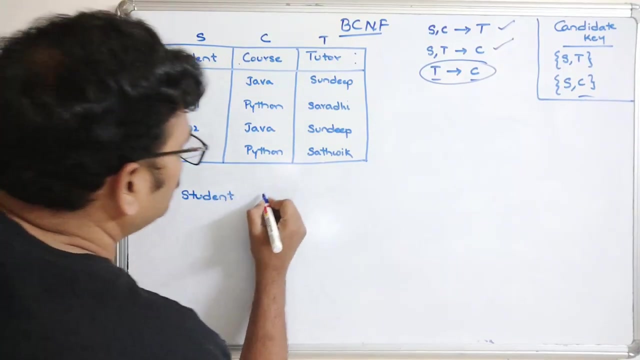 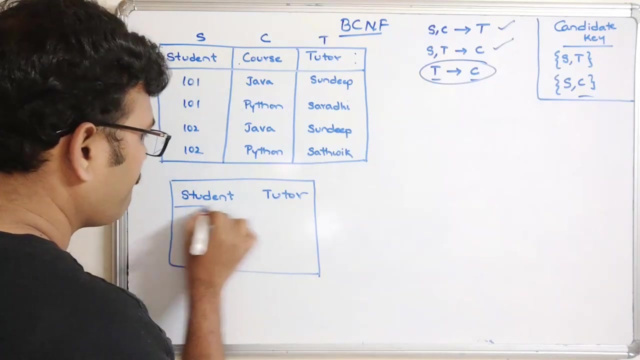 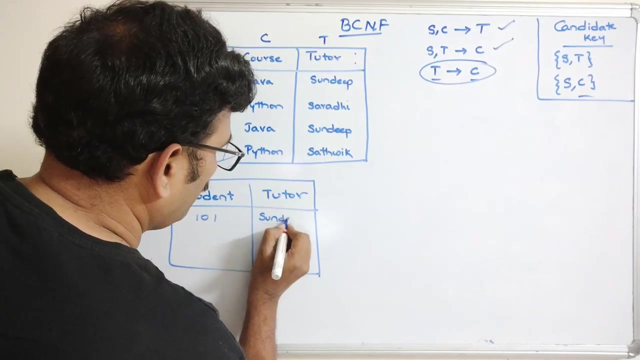 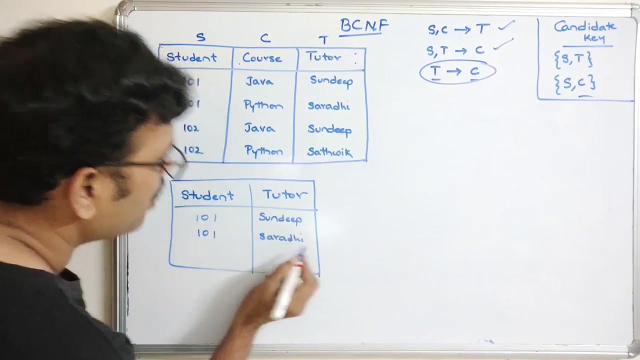 relation is not in bcnf, we have to decompose the relation. okay, we have to decompose the relation so so that it satisfies the BCNF. So how the relation should be decomposed and this relation can be divided into two relations, So one with student and a tutor. so student 101, Sandeep 101, Saradik 102, Sandeep 1002,. 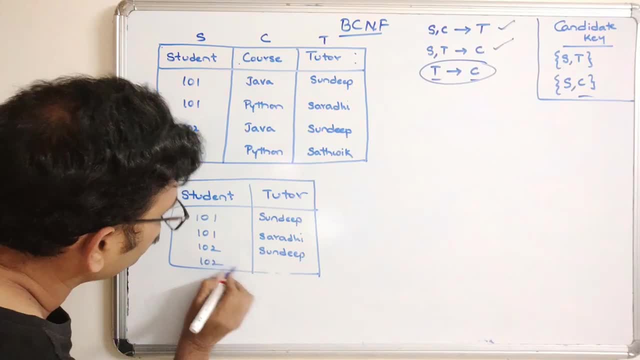 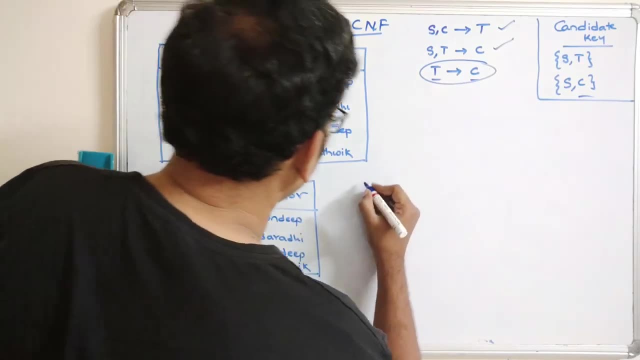 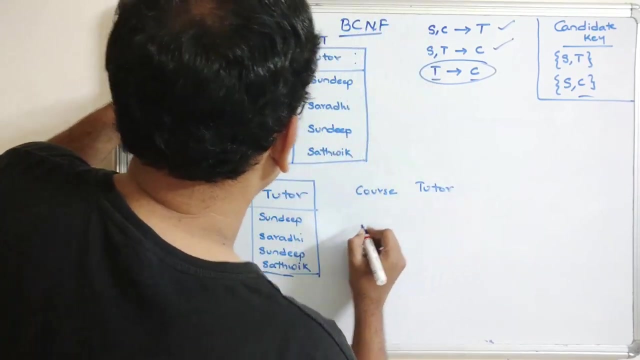 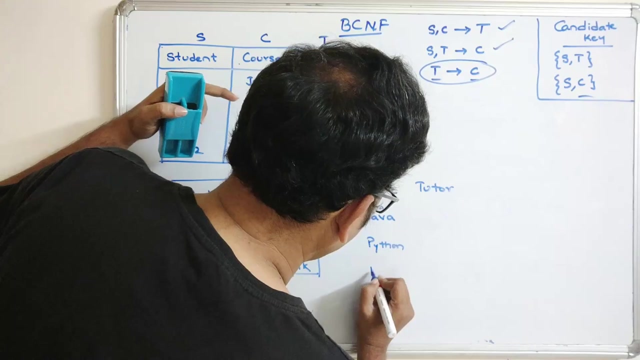 Saradik and 102, Saradik And the second relation course and a tutor. So course is Java, Python and Python, So Java with a Sandeep. Saradik and 102, Saradik and 102, Saradik and 102, and the second relation.